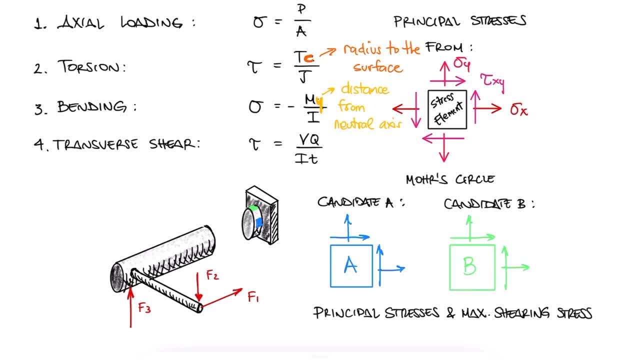 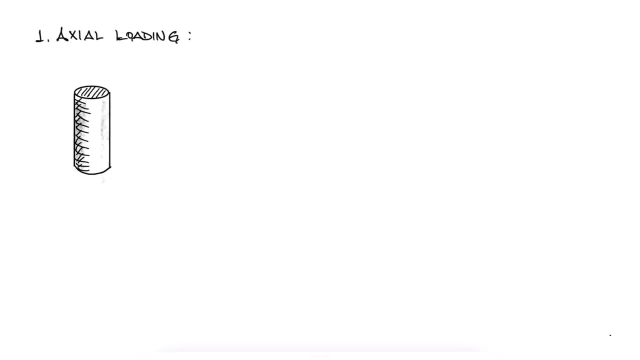 occurs. Additionally, the critical location candidates are usually located as far away as possible from the external loads that cause the moment that causes bending. but more on that later in this video. So let's begin with axial loading When a structure is subjected to direct compression. 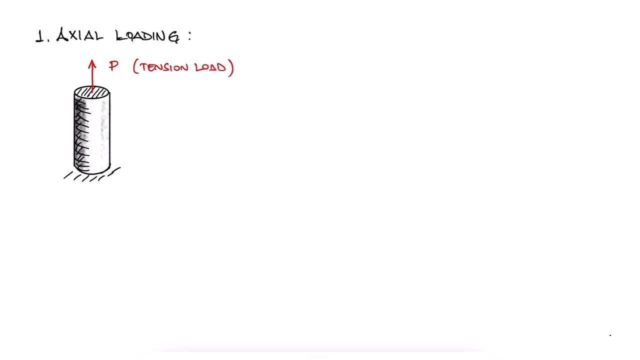 or tension. the location of the stress element doesn't make much of a difference, as long as the element is reasonably away from the external load. Performing a cut at the location of the stress element allows us to see a free body diagram of the top part and therefore 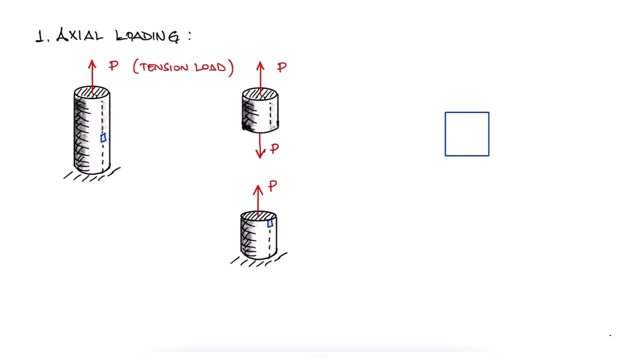 the reaction force of the bottom part. A normal load, that is, a perpendicular load affecting the action area, will produce a normal stress that we defined early in the course as the axial loading normal stress and in this case, any other element on the surface or not located. 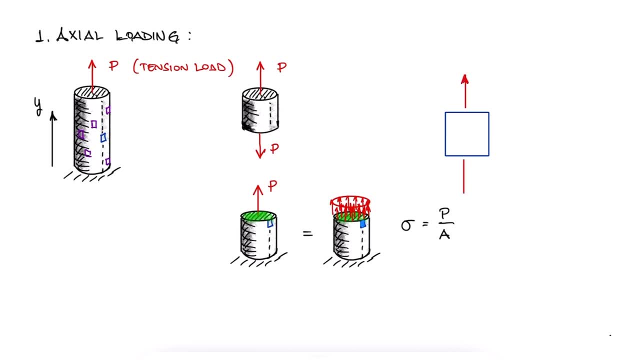 at any distance along the y-axis from the floor will be subjected to a σy that is equal to this axial external load P over the cross section of the structure at the location of the stress element. Any internal force at the location of the stress element, that is: 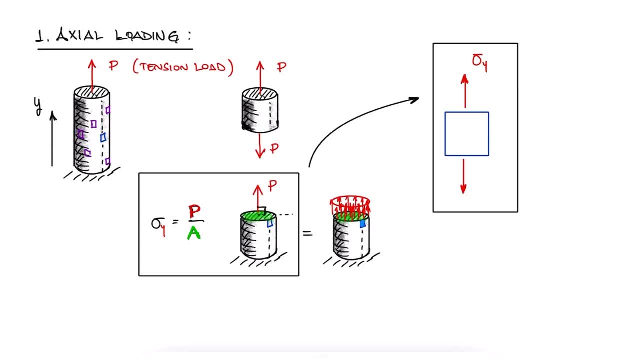 to the cross-section area will create a normal stress that is, either a compressive or a tensile axial stress, depending on the direction of the load. And remember that the cross-section area shape can be anything other than a circle, and the process still holds true Moving on to torsion. 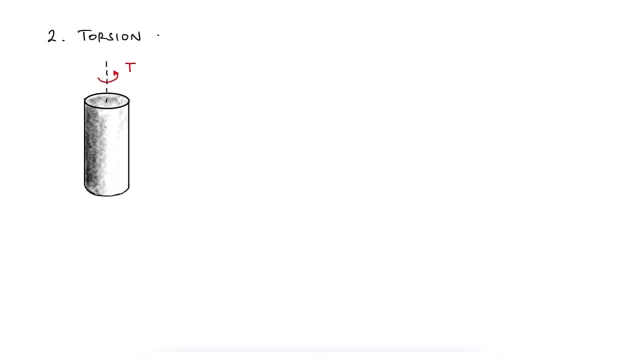 and in this case we do want a circular cross-section so that the polar second moment of area is easier to calculate. we see that the location of the stress element can once again be located anywhere along the y-axis, with the slight difference that in this case we need it. 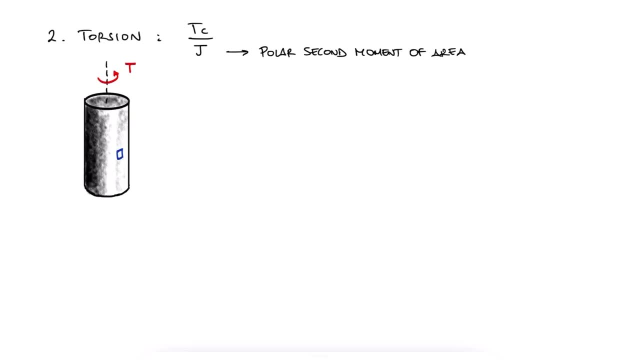 to be on the surface of the structure. This becomes apparent after we perform the cut of the structure at the location of the stress element. complete the free body diagram of the top portion, find the reaction couple for the bottom section and look at the stress profile. 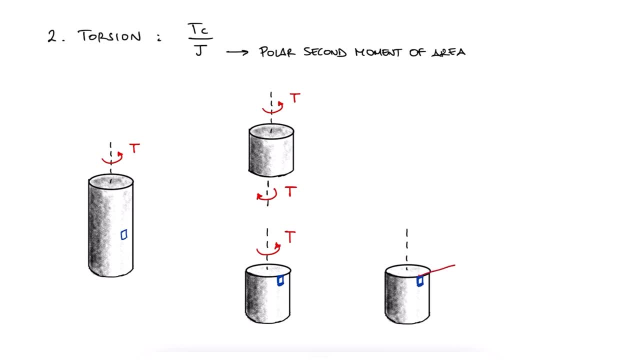 that this twisting couple, or torque T, is creating on the surface of the cross-section area. By looking at this stress profile from the top of the cross-section area, we see that only stress elements on the surface of the structure and regardless of their y-position, since the internal torque doesn't change along. 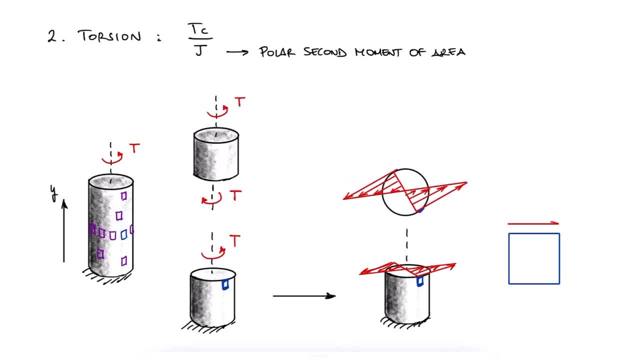 the y-axis will experience the same shearing stress: tau xy. Of course, since this stress element is not translating towards the right of the screen, we know that the bottom side is subjected to a vector equal in magnitude and opposite in direction. Additionally, since the 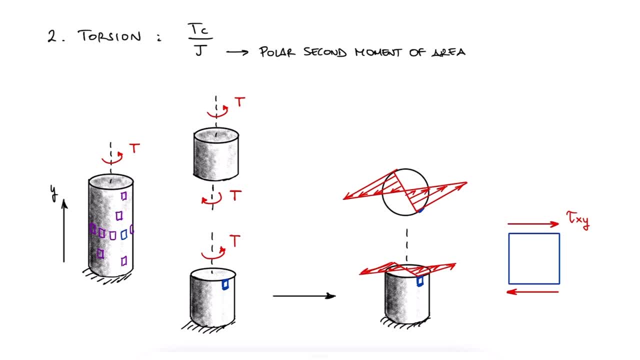 stress element is not rotating close to the surface of the structure. we can see that the top surface of the structure is subjected to a vector equal in magnitude and opposite in direction. By looking at the stress values of the cross-section area, we know that the vertical sides are subjected. 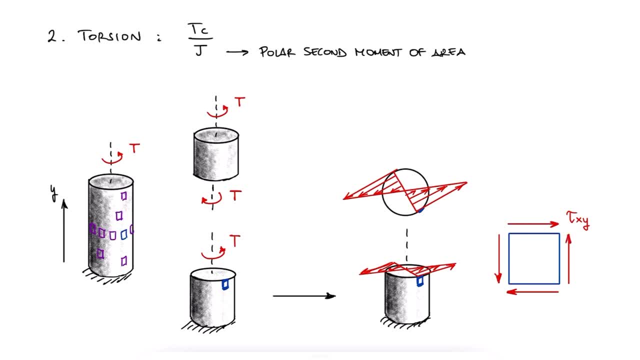 to stress vectors that counteract that clockwise rotation. The shearing stress value of tau xy would be equal to Tc over j in the direction shown, direction which is easily identified by bringing the internal torque T closer to the surface of the cross-section area. C would be the radius of the 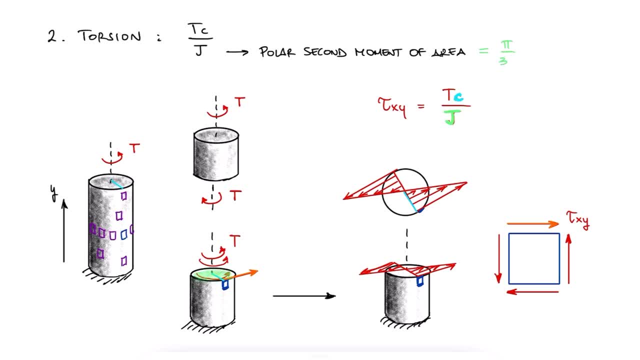 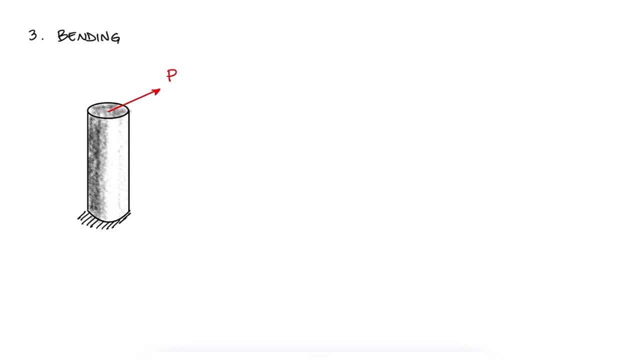 rod and j, the polar second moment of area of the cross-section area For the normal stress due to an external load. the location of the critical stress elements will be more limited. We know that elements located at the neutral axis will be subjected to a stress of zero. 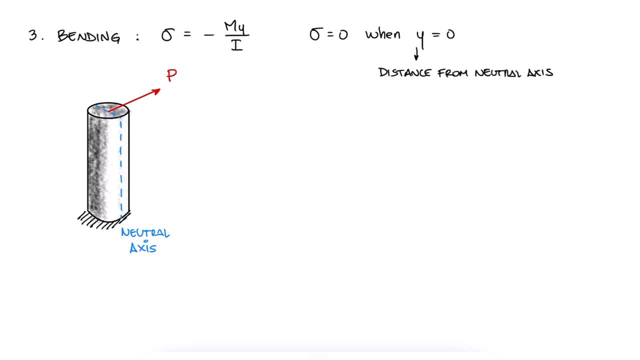 since the distance from the neutral axis to that location is also zero. The highest normal stresses will therefore occur when farthest away from the neutral axis. Tension for the green line we see and compression for the line opposite to it. Additionally, the magnitude of the internal 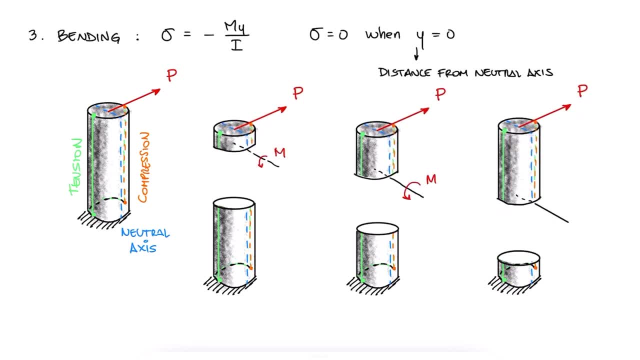 moment will increase and the stress value of tau xy will increase. and the stress value of tau xy will increase As we move away from the external load P. this internal moment increases because this is the moment that counteracts the couple produced by the load P multiplied by the perpendicular distance y. 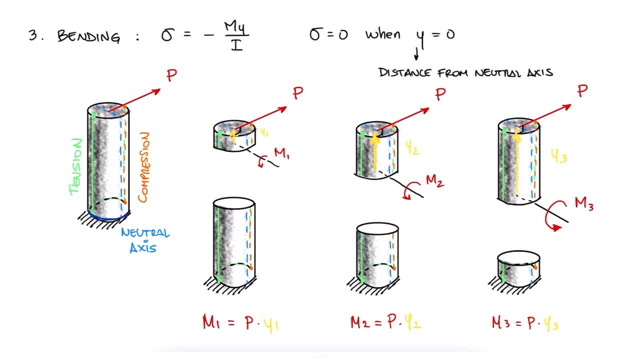 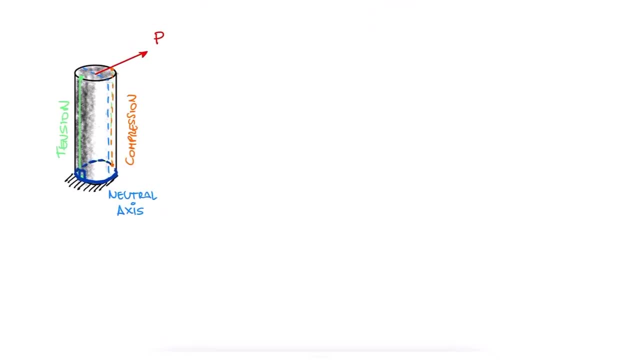 For this reason, we know that the critical location of the stress elements are located at the bottom, right next to the floor. green for tension and orange for compression, Performing the cut as far away as possible from the external load. P we see the same internal. 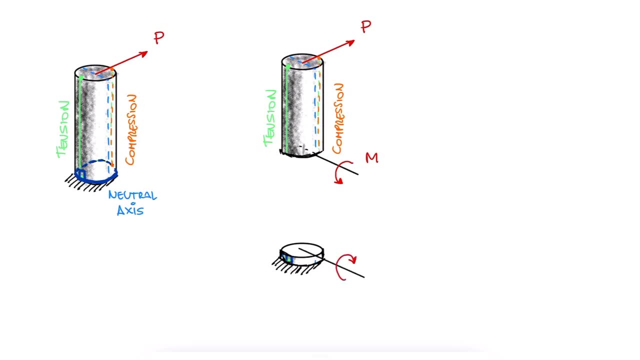 moment on the top section and its reaction internal moment on the bottom section. The value for this moment will be equal to P times the length of the rod, and by moving the moment vector notation closer to the surface of the cut we can easily identify that the element we see 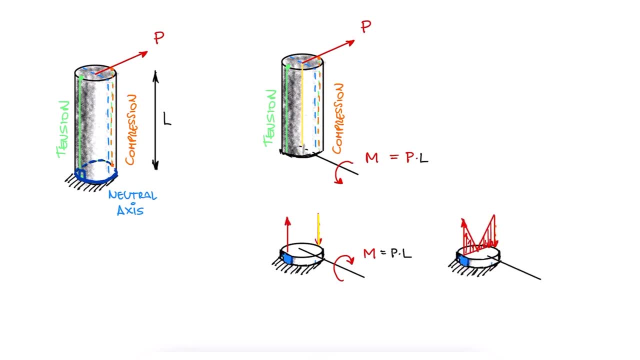 is in fact under tension and the one we can't see is under compression. Therefore, the stress element under tension would have a tensile normal stress in the vertical direction and the stress state at the back would have a tensile normal stress in the vertical direction and the stress state at 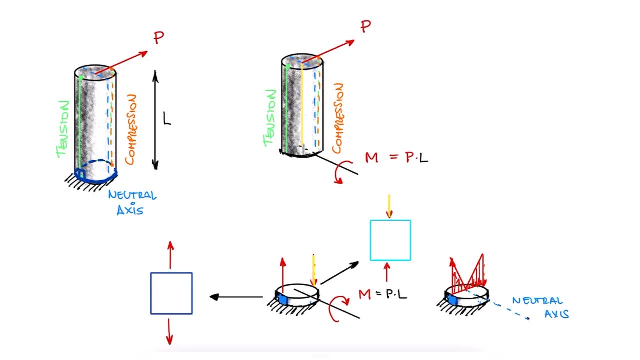 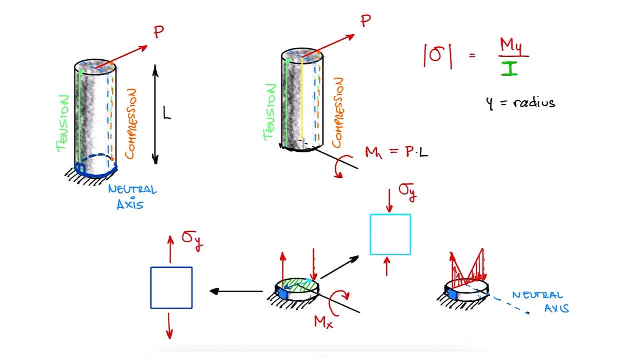 the back would have a compressive normal stress in the vertical direction. The magnitude of these stresses would be m y over i, where y is the distance from the neutral axis to the location of the stress, i the second moment of area of the cross section and the sub indices of sigma and m. 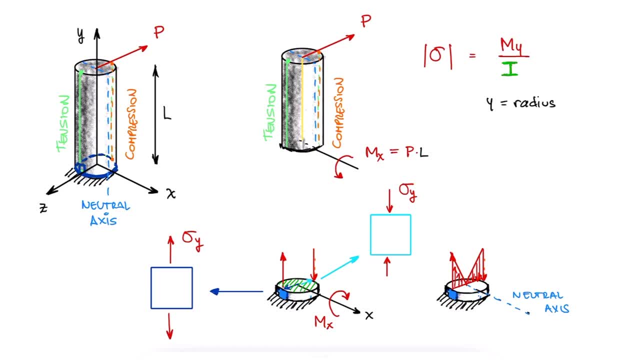 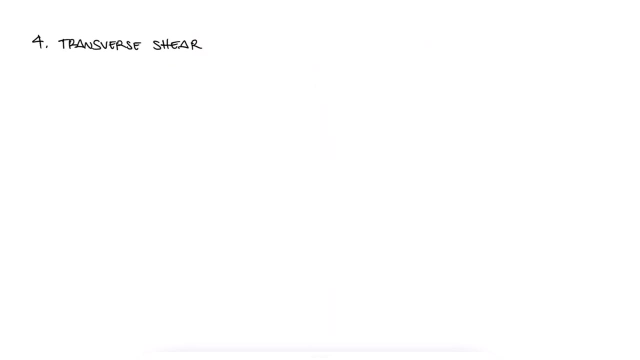 will depend on the coordinate system. Remember, for example, that a moment caused by a load on the z-axis at a perpendicular distance on the y-axis produces a moment about the x-axis. Therefore, m- x. Finally, for transverse shear, shearing stresses- we see that the location of 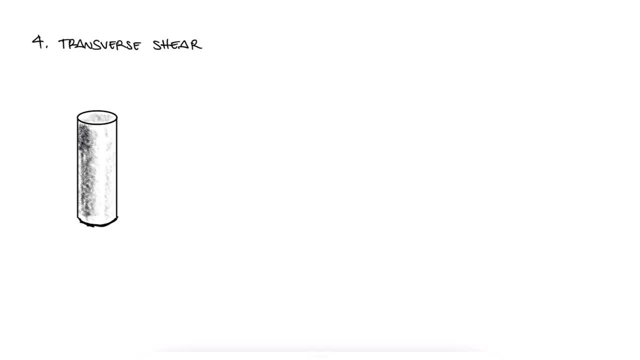 the stress elements follow some general rules that are almost the opposite to the bending rules, where the vertical location doesn't affect the internal shear force V, but because of the transverse shear stress profile, which shows decreasing stresses as you move towards the edges. 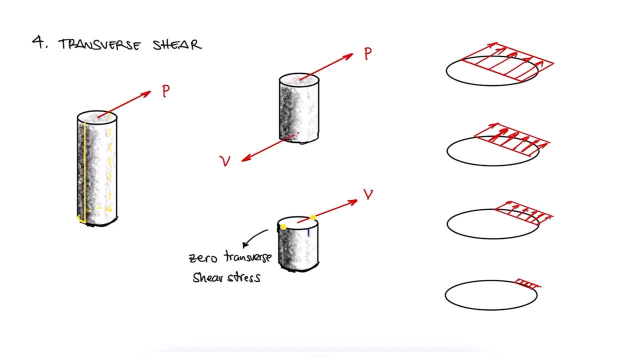 we know that there's two locations of zero stress and two locations, at least on the surface, where the transverse shear stress is at equality and the force in those most of the individual stress sacarreors, On the other hand, extreme in a situation like that where the stress is generally thought to come from electronics or checking and 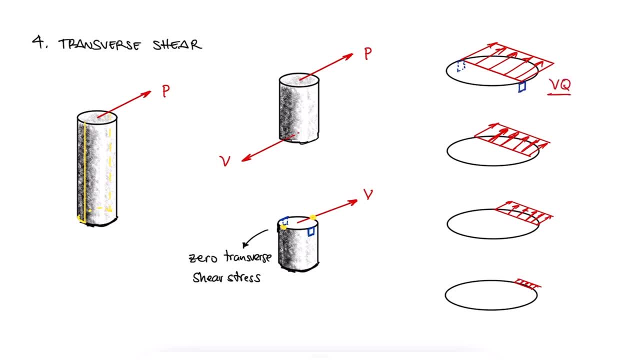 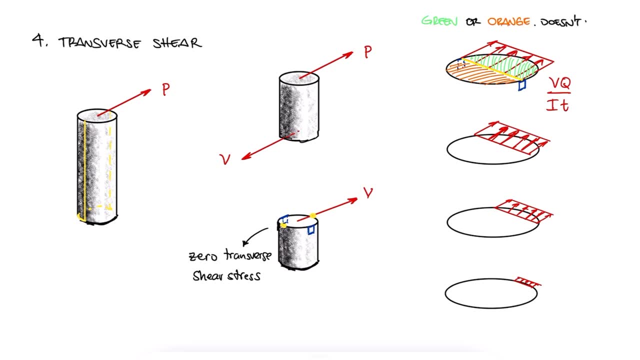 71, 4 c or thermal or other digital sensors we can să. Yeah, I'd say oh, absolutely maximum. The magnitude of the stress will be VQ over IT, where Q is the first moment of area of either side of the cross-section area from the location of the stress element, I, the second. 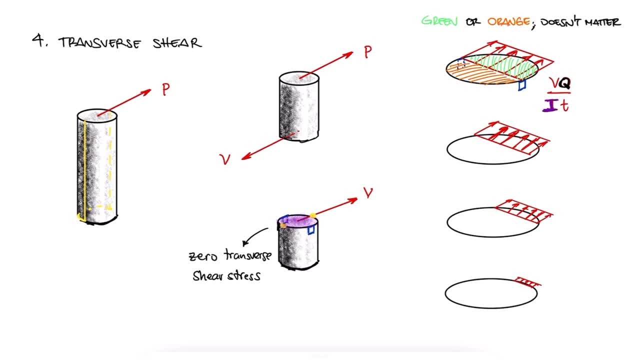 moment of area of the whole cross-section area and. T, the thickness perpendicular to the shear force at the location of the stress element. The direction of this shearing stress on the stress element is in the direction of the shear force. V- The direction of the other three vectors. 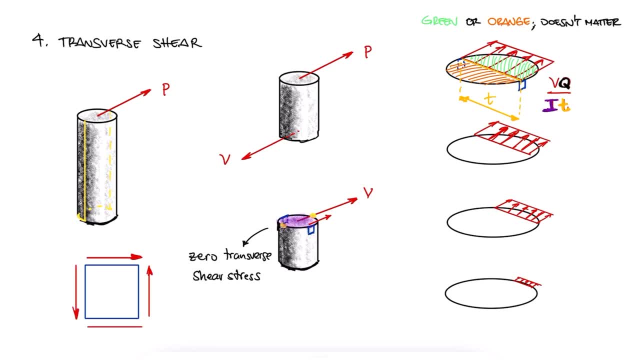 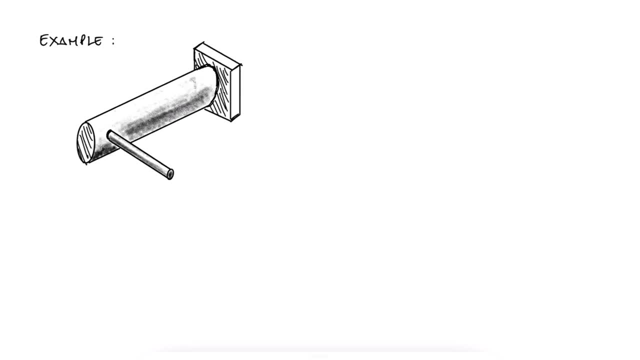 is found using the same logic we used before for torsional stresses. Let's look at a simple example where we want to find the stress state for the stress element shown due to the vertical external load P For the given coordinate system. we'll look at our stress element with the positive Z. 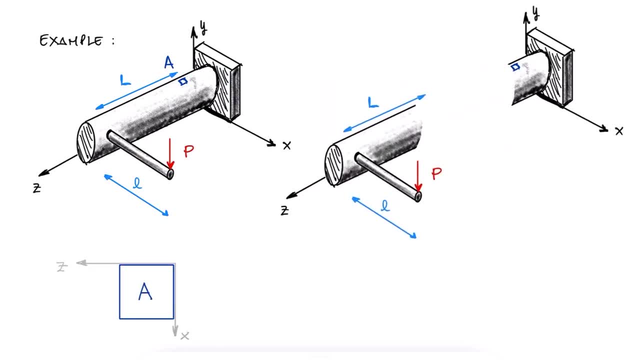 axis pointing left. By performing a cut at the location of the stress element, we see that there needs to be a reaction load in the positive Y direction and since this force is parallel to the cross-section area, not perpendicular or normal, we'll call it V a shear force For the section with the